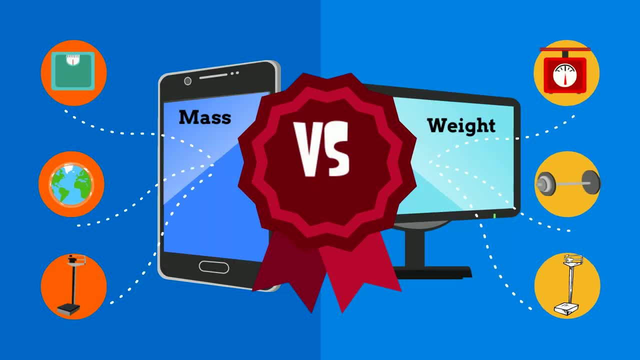 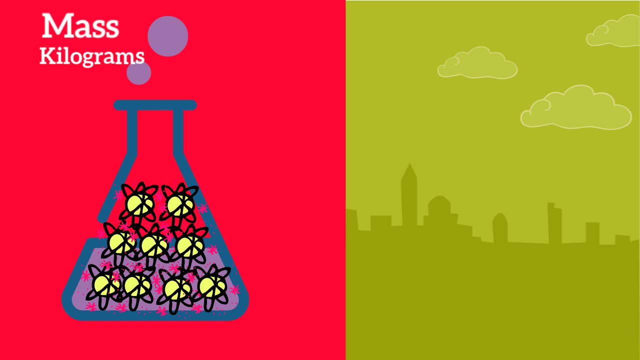 Welcome to MooMooMath and Science in Mass vs Weight. Isn't mass and weight the same thing? Not really. The mass of an object is the amount of matter an object contains, While weight is the force of the gravitational attraction the object feels. 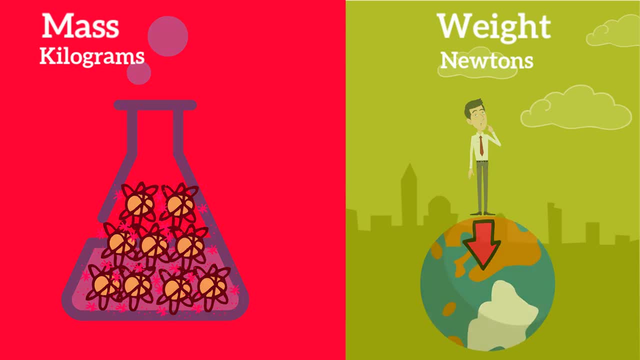 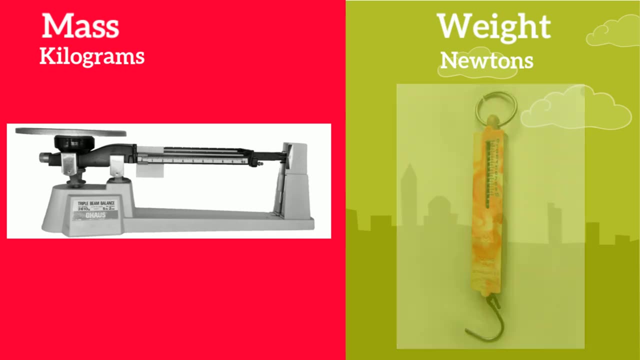 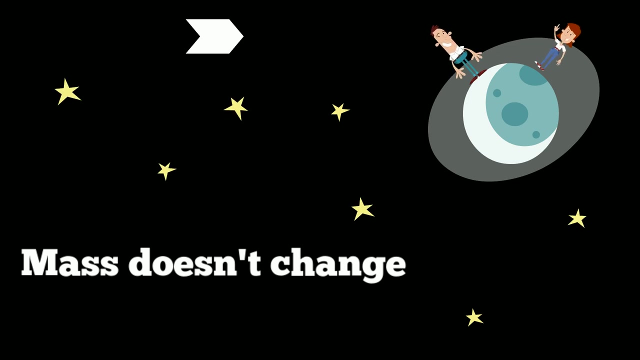 towards another object, like the Earth's center. Mass is measured by using a balance comparing a known amount of matter to an unknown amount of matter. Weight is measured on a scale. The mass of an object doesn't change. when an object's location changes Weight on the other. 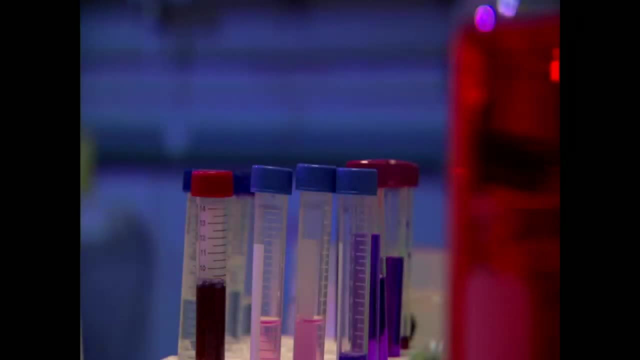 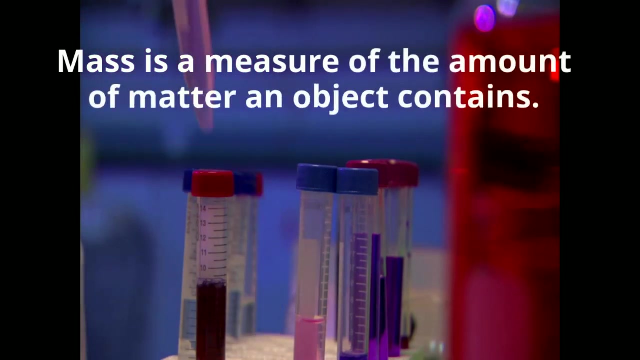 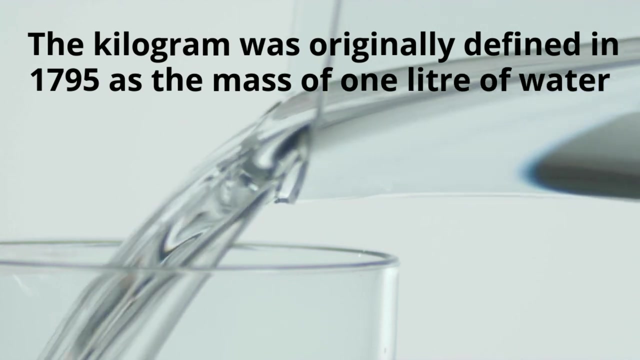 hand, changes with location. The mass of an object is a measure of the amount of matter in it, or in other words the amount of stuff it contains. The SI unit for mass is the kilogram. The kilogram was originally defined in 1795 as the amount of mass of one liter of water. It has since changed. 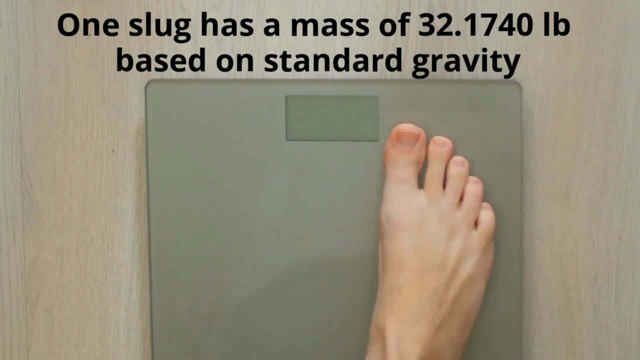 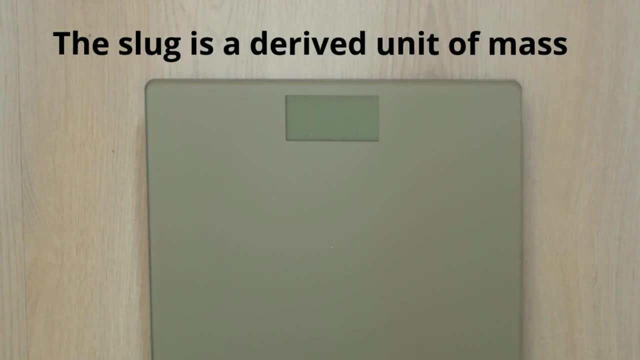 If you use the imperial system, the unit for mass is the slug- Yes, the slug, which has a mass of 32 pounds. So if you weigh 161 pounds on earth, your mass is five slugs- Yes, slugs. Weight is a measure of the force that gravity is pulling on the object. Gravity is a force, and 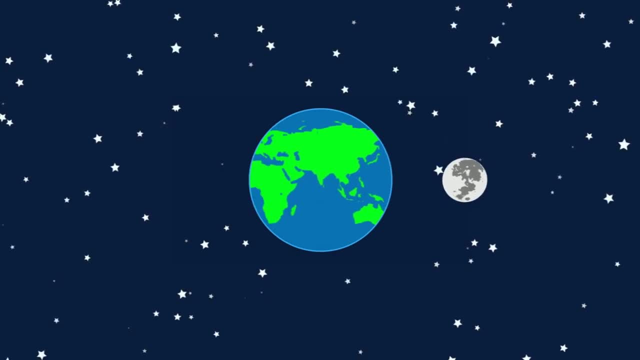 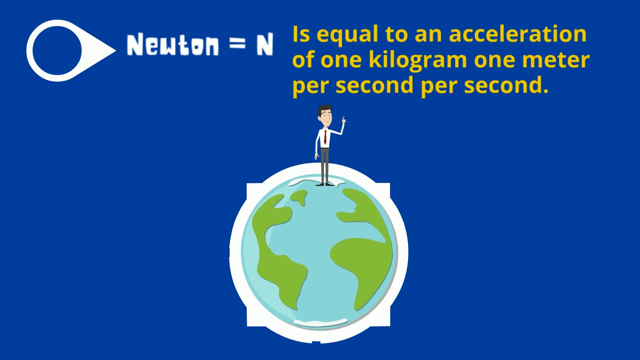 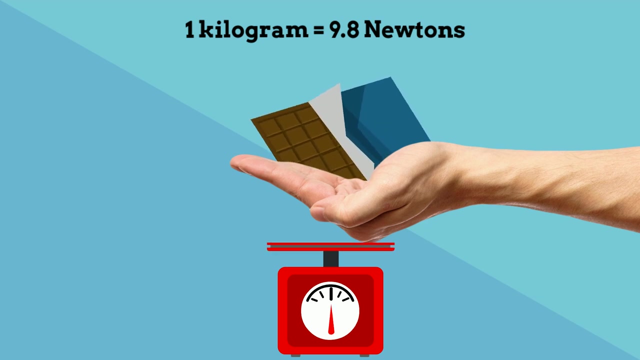 therefore, weight technically should be measured in newtons. A newton is equal to the acceleration of a mass of one kilogram one meter per second squared. For an example, let's take an object with a mass of one kilogram. It has a weight of about 9.8 newtons on the surface of the earth. 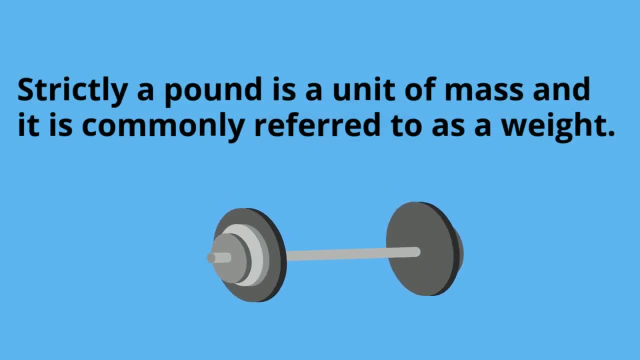 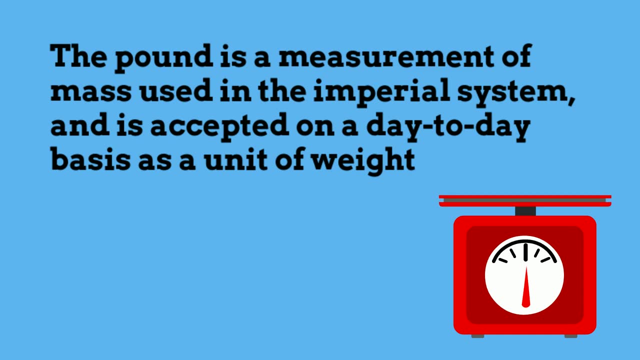 But here's where it may get a little confusing. There are other units that are used to describe weight that sound like mass. The imperial system uses the pound to measure weight and it's defined in terms of the kilogram as exactly 155359237 kilograms. Your weight can change based on the gravitational pull. Your weight varies on the moon and other planets, but your mass remains the same. If a cube has a mass of 90.91 kilograms and a weight of 200 pounds on earth, it will weigh 32 pounds on the moon, but still has a mass of 90.91 kilograms On Mars. the cube would weigh 76 pounds.